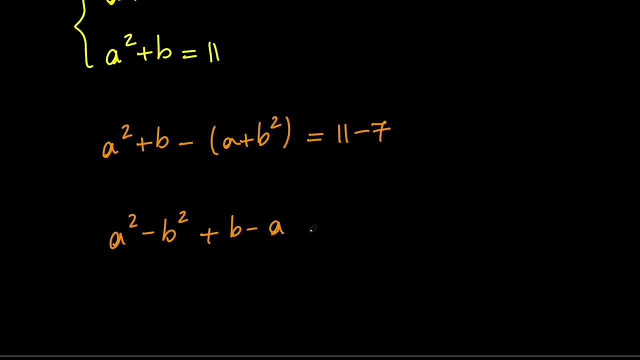 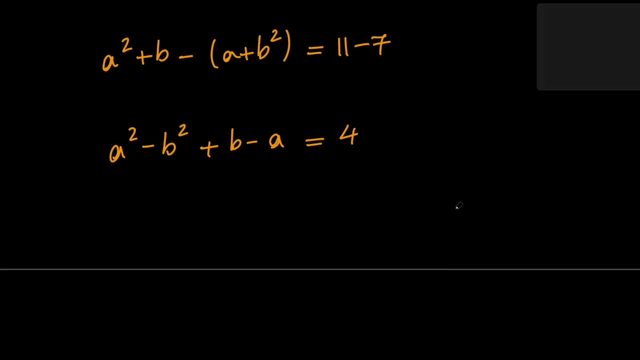 squared Plus b minus a and this equals 4.. Next, notice that a squared minus b squared is a difference of two squares, So we can factor this into a minus b times a plus b, And we can go ahead and take out a negative out of b minus a. So we're going to get minus the quantity a minus b equals. 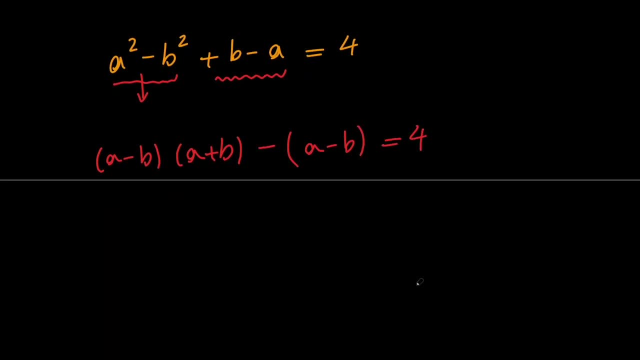 4. In this case, a minus b is the common factor, So we can pull it out and we'll have a minus b times a plus b minus 1 equals 4.. Now, since we want to solve for integer solutions and 4 can be written as: 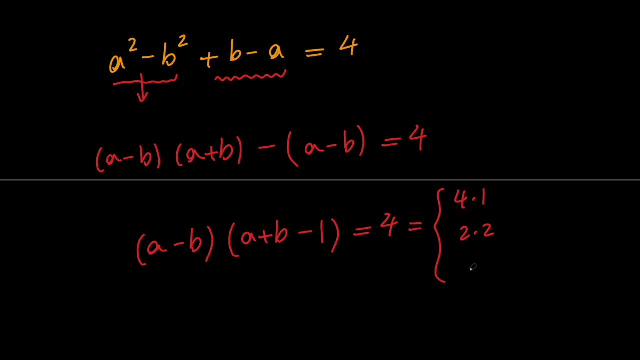 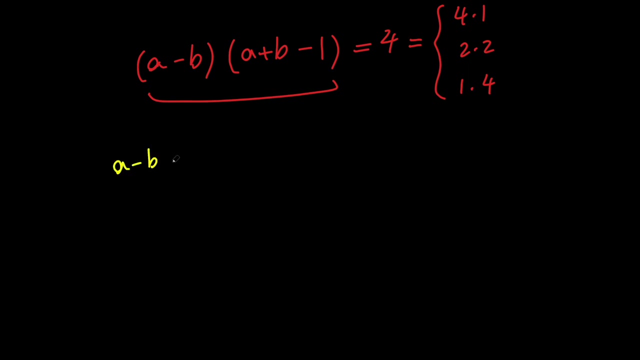 4 times 1, or 2 times 2, or 1 times 4, we have three cases for the values of these two factors. So in the first case we can say that we have a minus b equals 1.. Actually, a minus b equals 4.. And 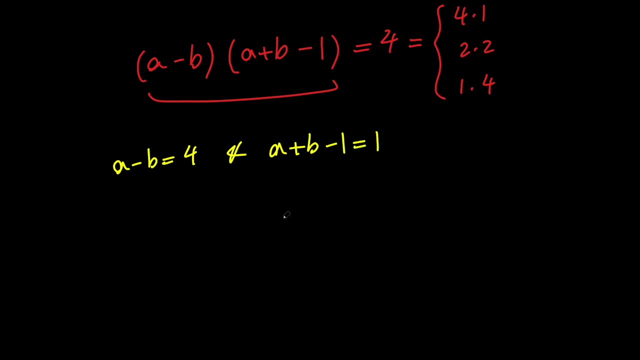 a plus b minus 1 equals 1.. And in the second case we have a minus b equals 2.. And a plus b minus 1 equals 2 as well. And in the last one we have a minus b equals 1.. And a plus b minus 1. 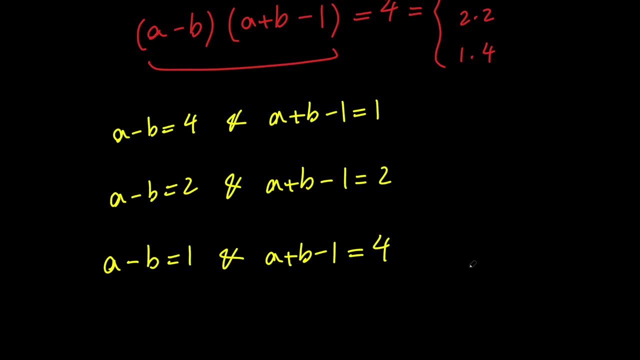 equals 4.. So let's go ahead and take a look at each of these cases and try to solve for a and b. So in the first case, if we go ahead and add one to both sides, we're going to get a plus b equals 2.. 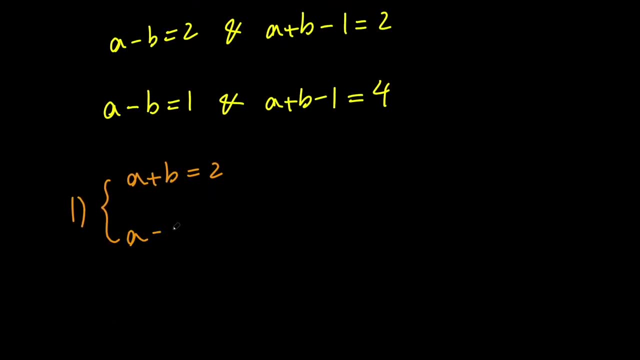 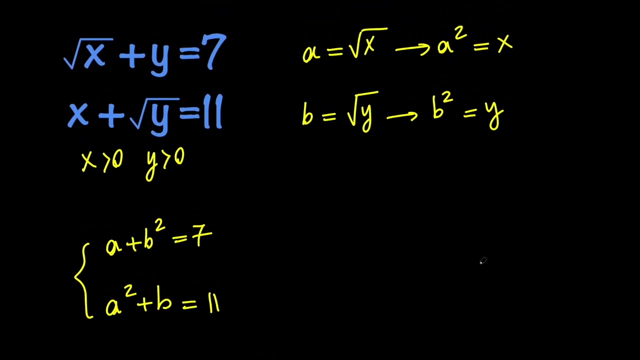 And we know that a minus b is 4.. So if we go ahead and add these two, we're going to get 2a equals 6, which means that a equals 3, and that means that b equals negative 1.. But remember that x and y are positive. actually, a and b are positive as well. 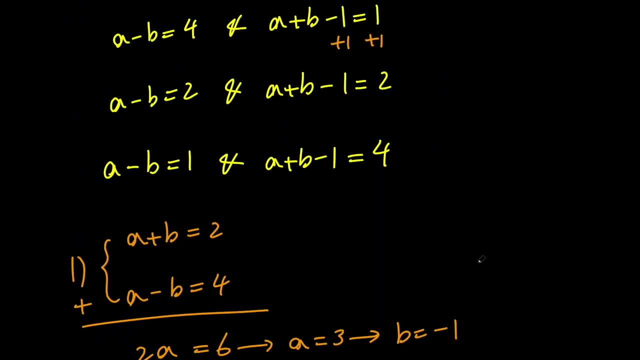 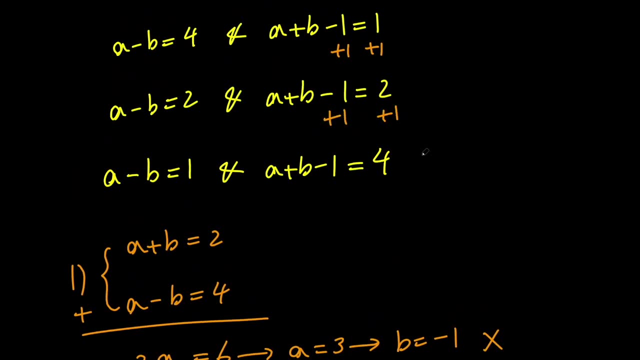 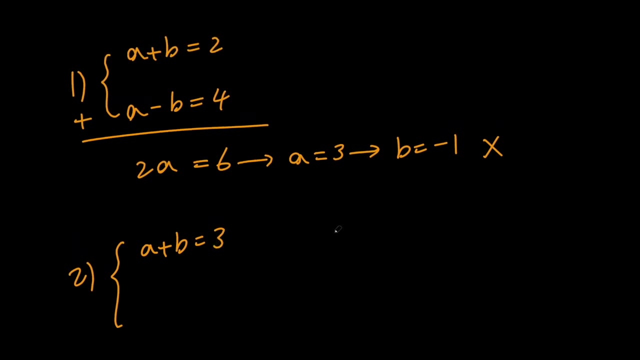 so that means that b cannot be negative and therefore this is not a valid solution. In the second case, if we add 1 to both sides, we get a plus b equals 3, so we have a plus b equals 3, and we have a minus b equals 2..